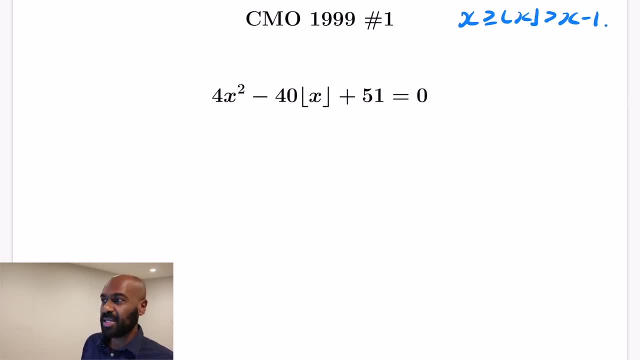 is that we can use that to get inequalities that x must satisfy if you rearrange the given equation. So the given equation says that 4x squared plus 51 is 40 times the floor of x. So using this inequality set of inequalities we just wrote down, you'll be able to find inequalities. 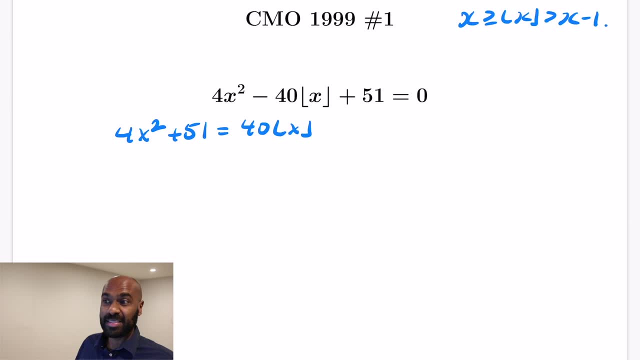 in that x must satisfy, which restricts the values of x that can satisfy them. So if you want to try that out, go ahead. this is a great time to by using those inequalities to figure out what values of x can even satisfy this equation, and then figuring out their floors to 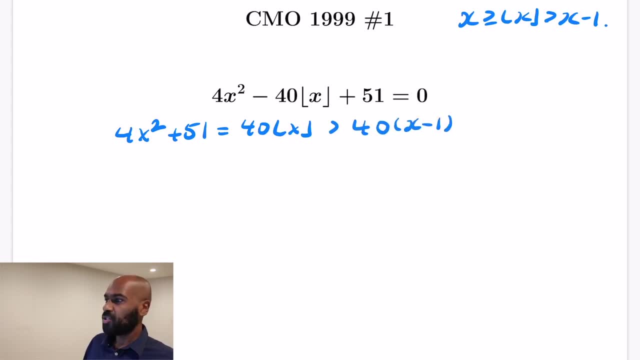 figure out what to do. Okay, so we're going to go ahead and do that. So, first of all, this quantity has to be strictly greater than 40 times the quantity x minus 1.. And if we rearrange this, this tells us that 4x squared minus 40x plus 91 is 40 times the floor of x plus 51.. So if we 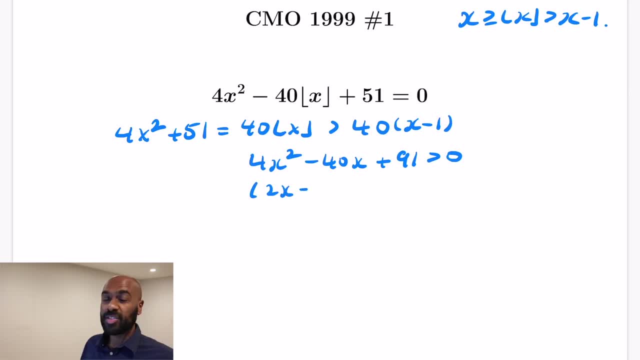 do that, we get 91 is greater than 0. Now, luckily, 91 is 37 times 13, so we can actually factor this into 2x minus 7 times 2x minus 13 being greater than 0. And that's satisfied. if we look at this, 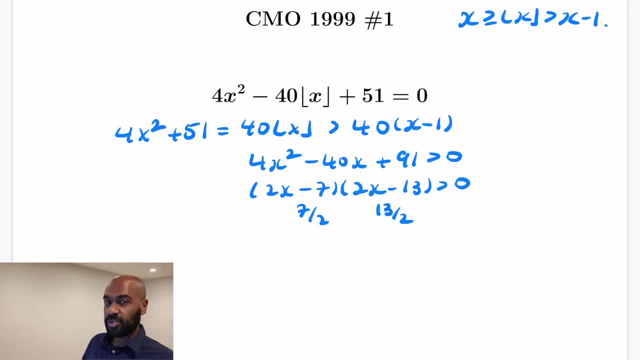 where the factors are 0, that's once we have 7 halves or 13 halves. so this strict inequality is satisfied for values of x that are strictly less than 7 halves, and that'll make both factors negative, and then when x is strictly greater than 0. So we can actually factor this into 2x minus 7. 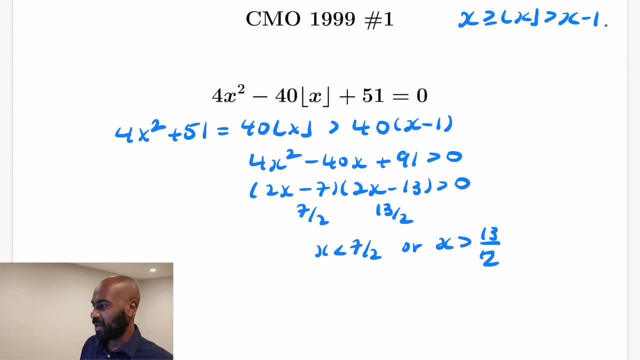 strictly greater than 13 halves, which will make both factors positive. Okay, so for x to satisfy that one inequality, we get these inequalities for x themselves. Now we have the upper bound that the floor of x is less than or equal to x. So 4x squared plus 51 is less than or equal to 40x If we rearrange. 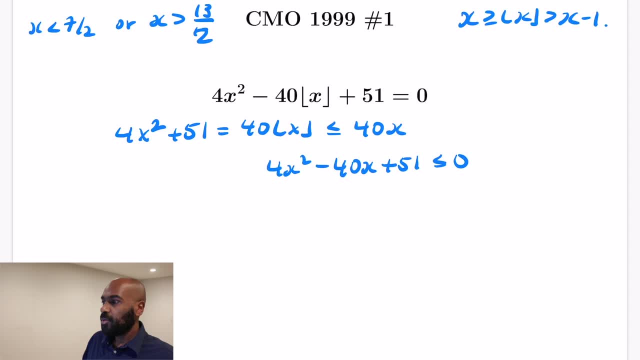 that gives us the following quadratic inequality: We can factor this as well, given that 51 is 3 times 17.. So we'll get 2x minus 17 as one of the factors, and then 2x minus 3.. We want that to be less than or. 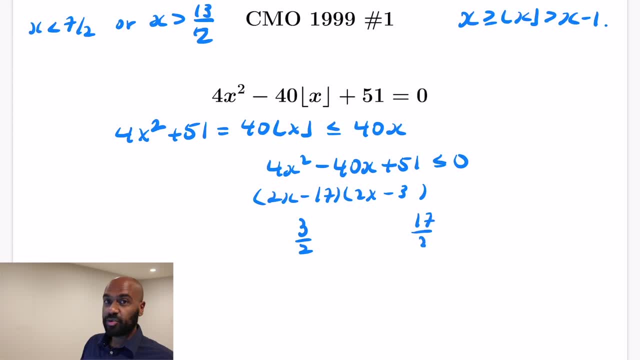 equal to 0. Now here the individual factors are 0 at 3 halves and 17 halves, and we want this quantity to be less than or equal to 0. so x has to be between those two quantities. So our values of x satisfy these two different sets of inequalities and if you merge them together that actually tells. you that 3 halves is less than or equal to x, and that's what we want. We want x to be 0 at 3 halves and 17 halves. So what we're going to do is we're going to multiply them, And we're going to multiply them by 8 and 7 halves. 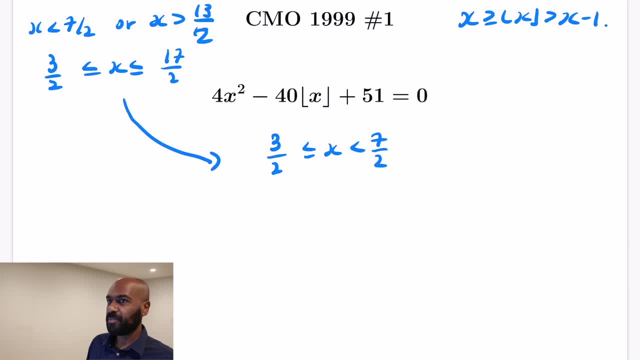 than or equal to x is strictly less than 7 halves, or that 13 halves bounds x, below which is less than or equal to 17 halves. So what we're going to do now, then, is take these two regions of x, which are relatively small, and look at what that forces floor of x to be, and then, once we have, what floor of 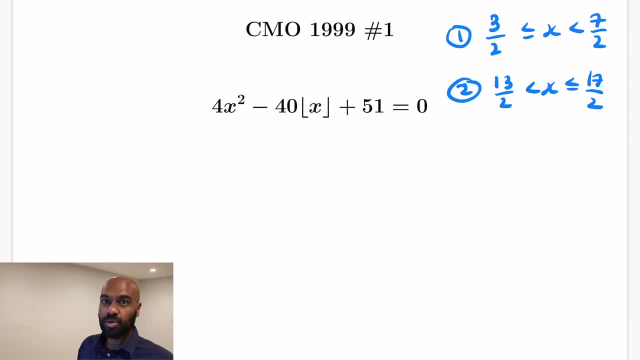 x is forced to be. we can go back to this seemingly quadratic equation and actually solve it to figure out if things work out. So in the first case, x is between 1.5 and 3.5, so the floor of x is going to be either. 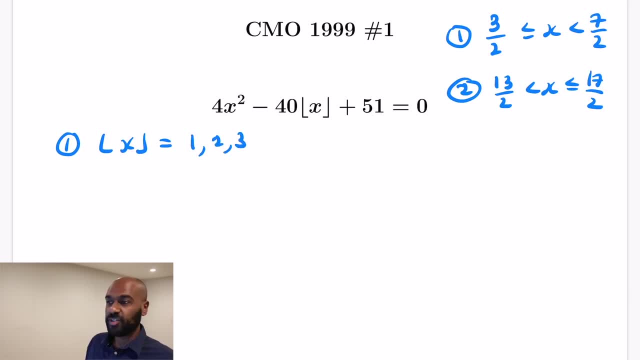 1 or 2 or 3.. So let's take each case individually and see what happens. If the floor of x is 1, then our equation becomes: 4x squared minus 40 is 15.. So 4x squared plus 51 is 40.. 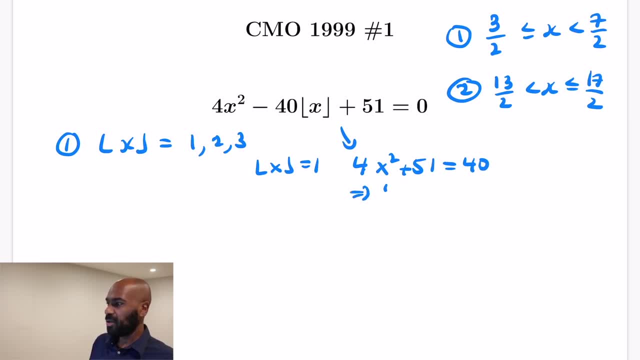 Okay, but if we rearrange that, that would make 4x squared a negative number, and that's not possible since we're solving for real values of x. So that rules out the case that the floor of x can be 1.. Okay, so then now let's move on to what happens with the floor of x being 2, and we see that. 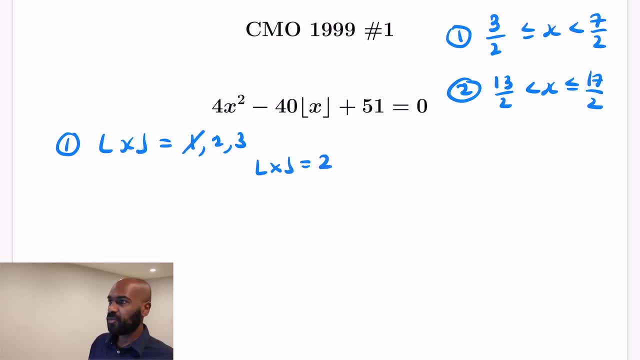 these situations are going to be particular and we need to check things. So if the floor of x is 2.. Our equation becomes: 4x squared plus 51 is 80.. Alright, rearranging, we get 4x squared. then is going to be the difference of 80 and 51. 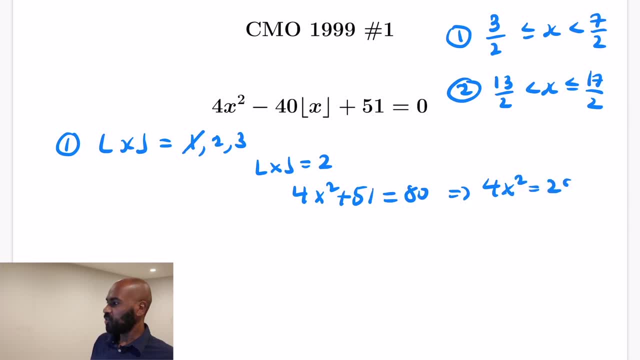 which is 29.. Alright, and so x, then, is going to be the square root of 29 over 4.. The reason we know that x has to be positive is because x is in the range between 3 halves and 7 halves. Okay, now we think we're fine, but the problem here is we've got to check that the floor. 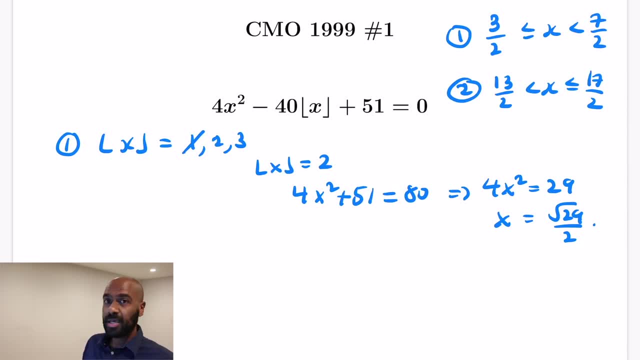 of x actually is 2.. That's the condition we mandated in this particular case. If it wasn't, then this actually doesn't work as a solution for this thing that we're looking at Now. the square root of 29 is between 4 and 6, because 29 is greater than 16 and 29 is 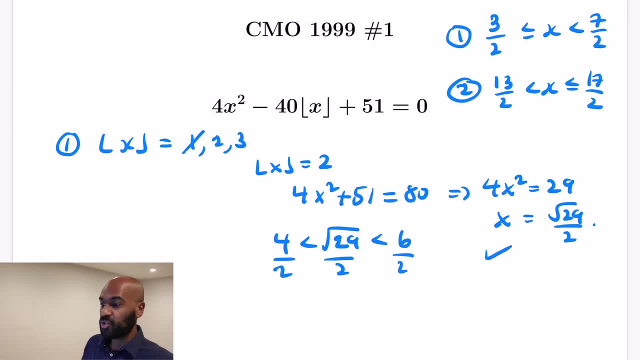 less than 36.. So the square root of 29 over 2 actually is between 2 and 3, strictly, so the floor of it actually is 2, and so we're fine and we'll record that as one of our possible solutions. Now let's move on to the floor of x is 3.. 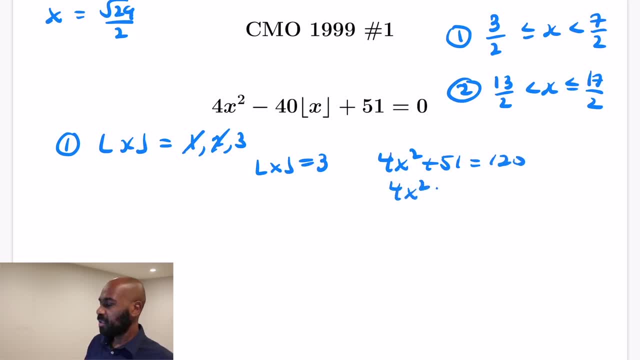 We got 4x squared plus 51 is 120 in that case. So 4x squared is going to be the difference of these two, which works out to 69, which gives us that x is the square root of 69.. All divided by 2.. 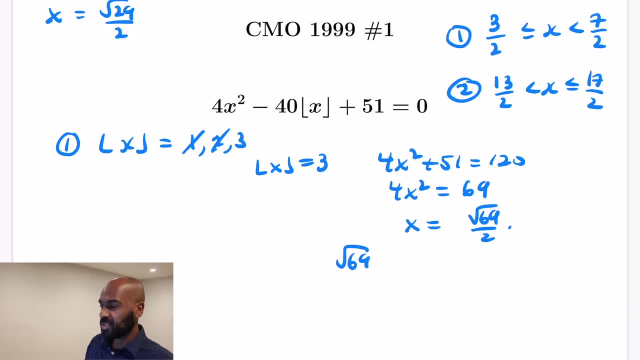 All right. so now again, is the square root of 69 over 2 actually a number whose floor is 3?? The square root of 69 is between 8 and 9, so if we divide these by 2, we get that actually the floor of the value x is actually strictly greater than 4.. 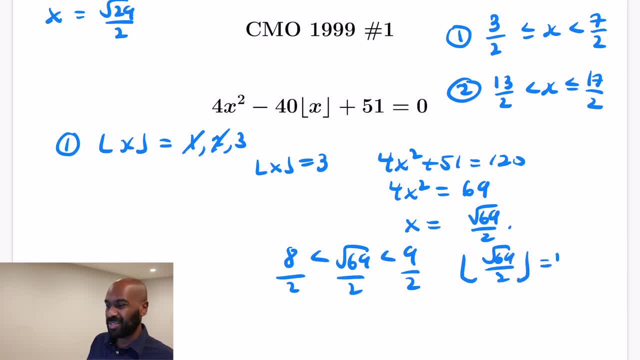 So the floor of it happens to be then 4, which is not the 3 that we assumed would be equal to. We gave a value for floor x, so that rules that out. Okay, so for the values of x between 3 halves and 7 halves, we only have one solution. 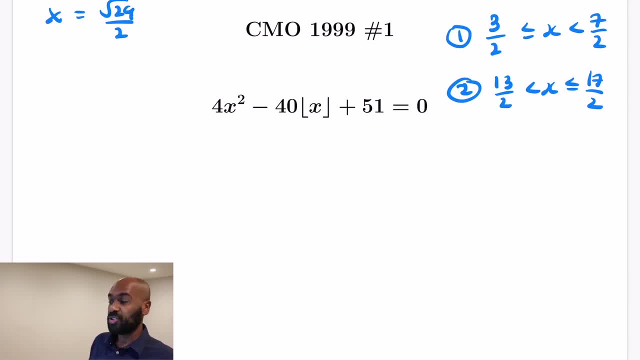 So now what remains is to check the values of x that are between 13 halves and 17 halves, doing the same type of process we just did with setting floor of x to values. Now, 13 halves is 6.5 and 17 halves is 8.5, so the possible values of floor of x here: 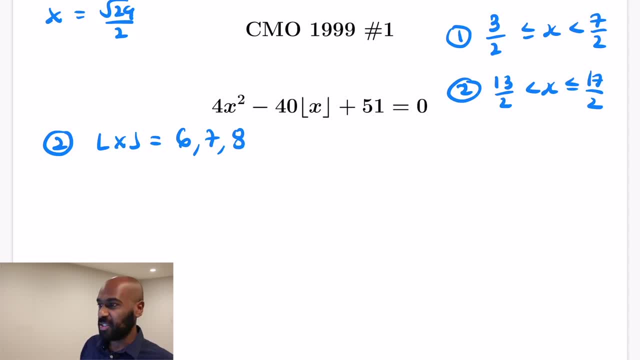 are 6,, 7 and 8.. So let's check each of these and see what happens. Starting with the floor of x being 6. we're going to play the same game that we did with the other values, but we need to make sure that things don't go awry. 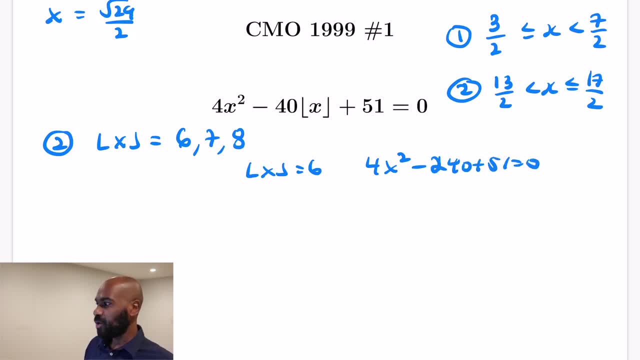 So here we get that 4x squared minus 240 plus 51 is 0.. Okay, so rearranging in this case we get: 4x squared is 189, and so x is the square root of 189.. All divided by 2.. 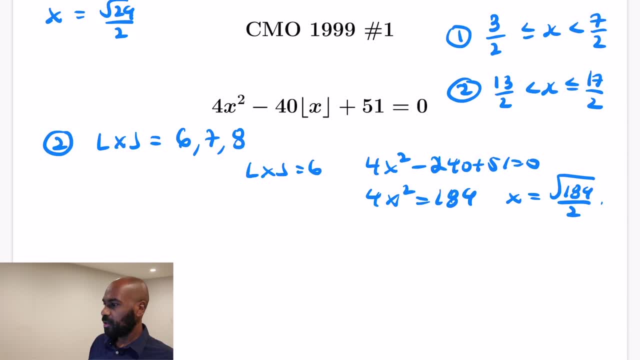 Okay. so this is where it's useful to have perfect squares in our mind and sort of know what they are. So 196 is a perfect square, it's 14 squared, and the square just below 189 is 144.. And so this value, the square root of 144, is 12, so we're lower bounded by 6, upper bounded. 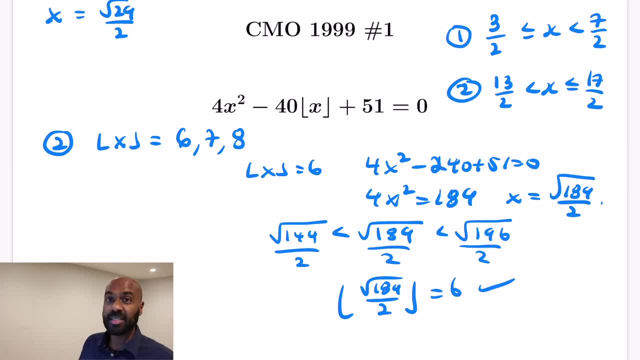 by 7 here, And so the floor of this actually is 6, and so we're happy. Okay, just two more values to check. First, the floor of x is 7, we got 4x squared minus 280 plus 51 is 0.. 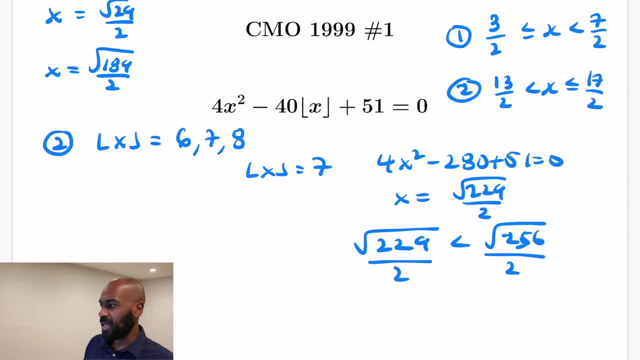 Now we did the math to figure out that that's the root of 229 over 2.. That's upper bounded by the root of 256 over 2, we don't even need a lower bound in this case. Um, so this upper bound is going to be 8.. 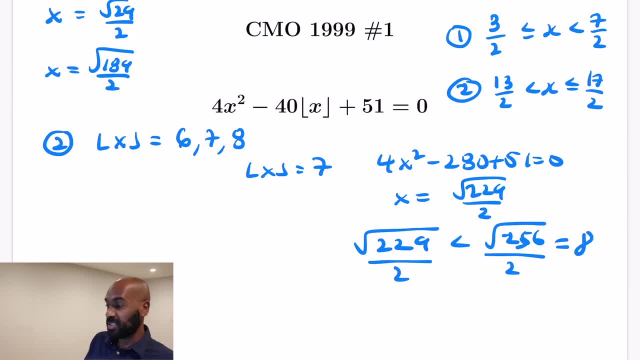 So we need a lower bound in this case. Um, so this upper bound is going to be 8.. So we know this thing is just below 8,, um, so the floor of it has to be 7.. Because 256 is the next perfect square after 229.. 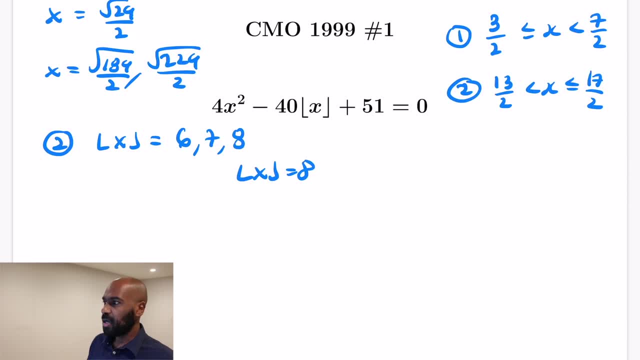 Okay, and finally, the floor of x is 8,. um, so in that case, uh, we get 4x squared minus 320 plus 51 is 0.. Okay, and so x squared then, in this situation, is the square root of 8.. 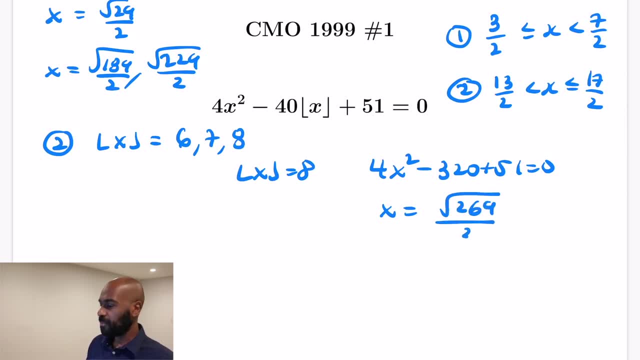 So we have 269 all over 2.. Okay, and by the same thing that we did before, the square root of 269, the next perfect square after 269 is what is it? it's 289.. That's 17 squared.